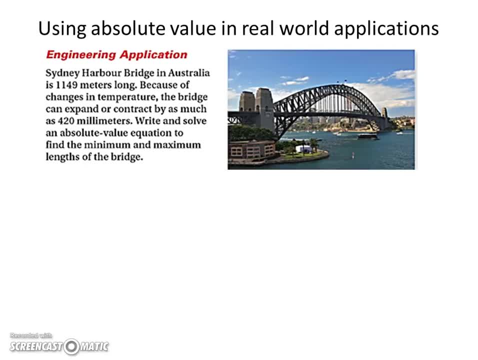 Australia is 1149 meters long. Because of changes in temperature, the bridge can expand or contract by as much as 420 millimeters. Write and solve an absolute value equation to find the minimum and maximum lengths of the bridge. Now, before we start, remember, guys, that the 420 is in millimeters and the length 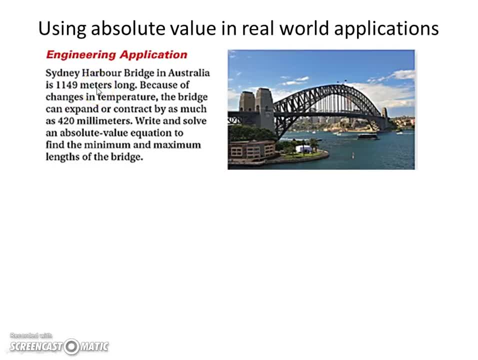 of the bridge is in meters. We want those to be the same, So millimeters we can write as meters by making this into 0.42.. So, with that in mind, our optimum value, what we want the bridge length to be, is 1149 meters. 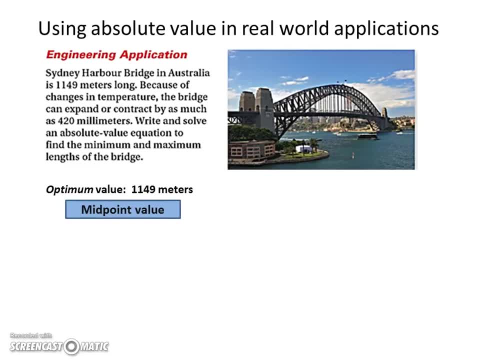 That's what we want the bridge to be, to be, And that's really, when we're talking about an absolute value equation, that's our midpoint value, That's what we want it to be, But we're allowing the bridge to vary by as much or as 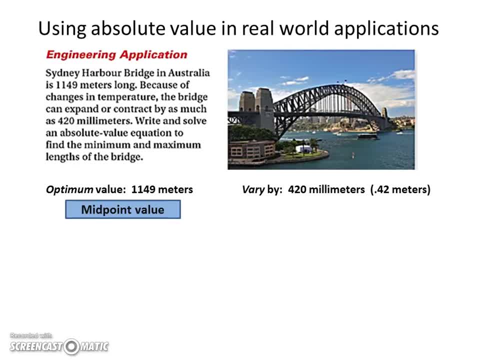 little as 0.42 meters, which is 420 millimeters, Because, remember, there's a thousand millimeters to one meter, So it's a little less than half a meter, Okay, and that's the distance from that midpoint value. So that's how much we're allowing it to be bigger or smaller. So if you think in 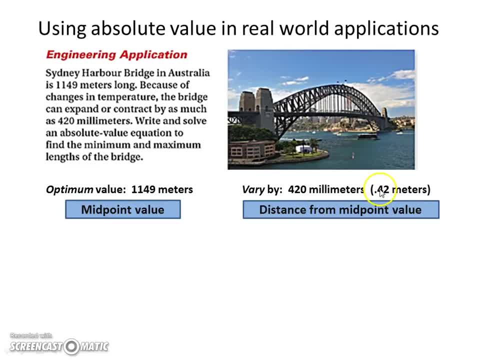 terms of a segment or what we've been doing in the past. we can go plus 0.42 or minus 0.42, if you think about it in terms of a segment. So our absolute value equation would be our x minus. 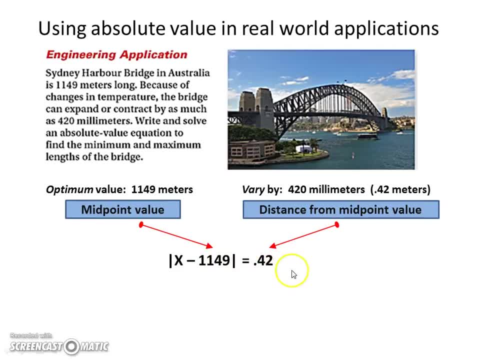 1149 equals 0.42.. Once again, this is what we want it to be, And this is how much we're allowing it to vary by Okay. so we're allowing it to vary by Okay. so we're allowing it to vary by Okay, so. 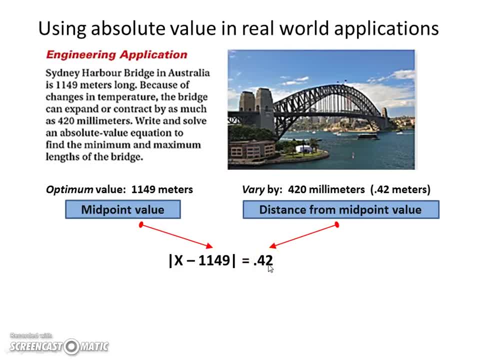 can go up or down by 0.42- same thing we've been doing, but now we're doing it with real-life problems. so obviously there's going to be two answers, guys: the minimum and the maximum. the minimum is going to be when we take away 0.42 or if. 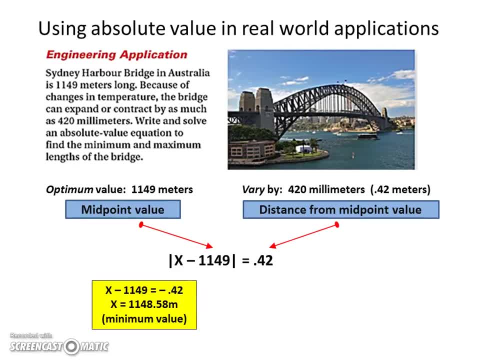 you think about it in terms of the segment drawing that we've been using when you're going to the left, right, and that would give you a total value of 1148.58 meters if we're going the opposite direction, to the right. in other words, we're making it bigger, we're allowing it to expand a little bit, then 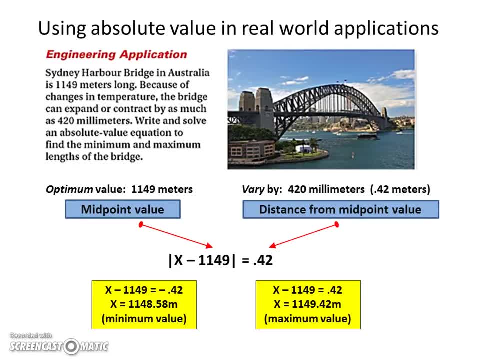 we're going to add that 0.42, so it's going to give us 1149.42 meters, not a lot of space, but we, we have to let the bridge allow to quote-unquote breathe, okay, and temperature changes make things expand or contract, and that's what's. 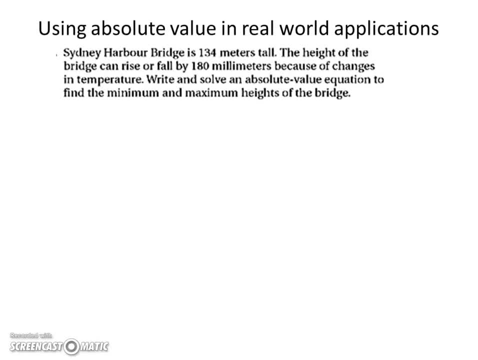 happening here, so let's look at another example. okay, so let's look at another example. okay, so let's look at another example. we're still looking at this bridge, but we're still looking at this bridge, but now we're looking at it expanding. and now we're looking at it expanding and 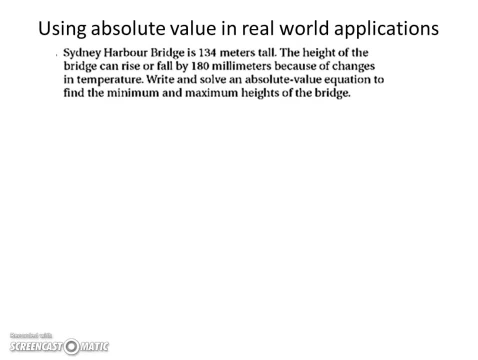 now we're looking at it expanding and contracting in a different way. it says contracting in a different way. it says contracting in a different way. it says the Sydney Harbor Bridge is 134 meters. the Sydney Harbor Bridge is 134 meters. the Sydney Harbor Bridge is 134 meters tall. so we're talking about a difference. 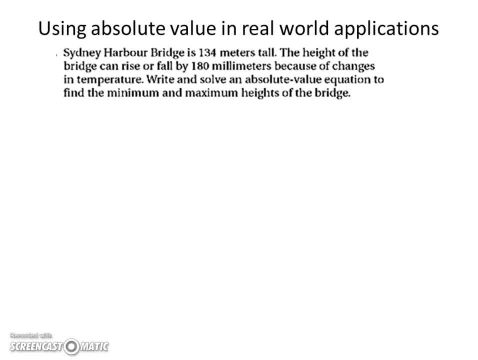 tall. so we're talking about a difference tall. so we're talking about a difference in height. the height of the bridge can in height, the height of the bridge can in height. the height of the bridge can rise or fall by 180 millimeters. because rise or fall by 180 millimeters? because 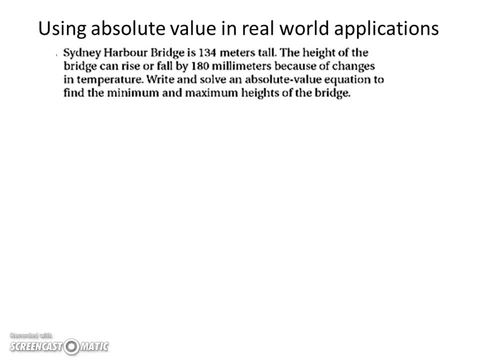 rise or fall by 180 millimeters because of changes in temperature right and of changes in temperature right and of changes in temperature right. and solve an absolute value equation to find: solve an absolute value equation to find: solve an absolute value equation to find the minimum and the maximum heights. so 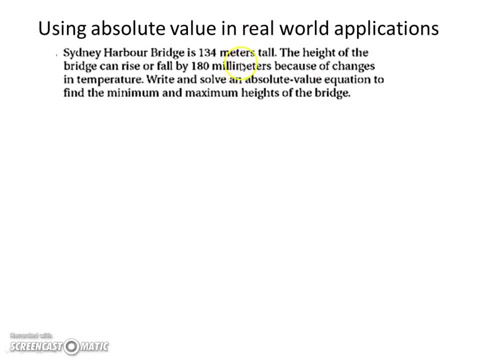 the minimum and the maximum heights. so the minimum and the maximum heights. so once again, you can see that we have, once again you can see that we have. once again you can see that we have meters and millimeters, so we want to. meters and millimeters, so we want to. 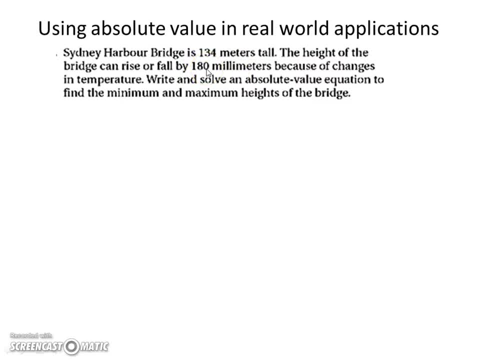 meters and millimeters. so we want to change this to meters, which would be: change this to meters, which would be: change this to meters, which would be point 1: 8. so we want the bridge to be point 1: 8. so we want the bridge to be: 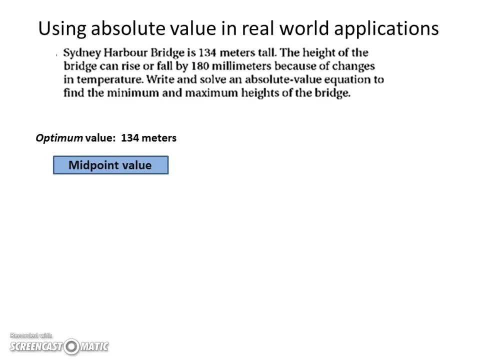 point 1: 8. so we want the bridge to be 134, that's the optimum value, and another 134, that's the optimum value and another 134, that's the optimum value. and another way of thinking about that once again. if way of thinking about that once again, if. 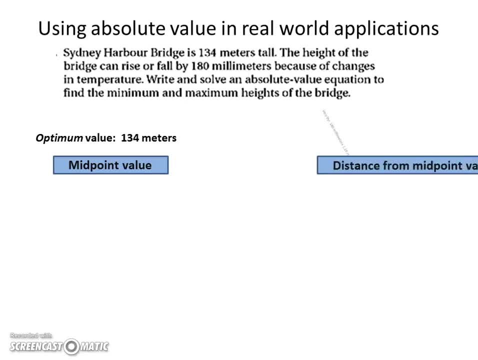 way of thinking about that. once again, if we're thinking about our segment, is that we're thinking about our segment? is that we're thinking about our segment? is that we can either make it point 1- 8 more, or we can either make it point 1- 8 more, or 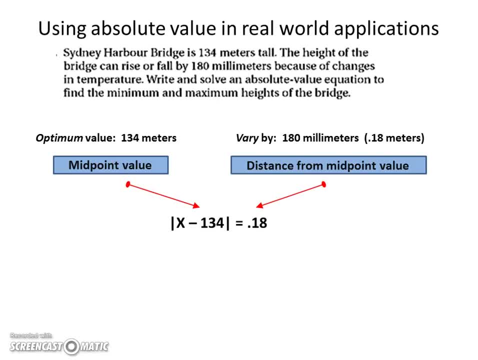 we can either make it point 1: 8 more, or point 1: 8 less. so there's our absolute point: 1: 8 less. so there's our absolute point: 1: 8 less. so there's our absolute value. equation: the 134 is the optimum. 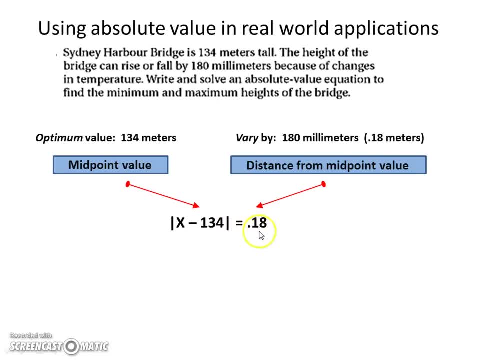 value equation. the 134 is the optimum value equation. the 134 is the optimum value. that's what we want it to be. but value, that's what we want it to be. but value, that's what we want it to be, but we allow it to vary by point 1- 8, so it 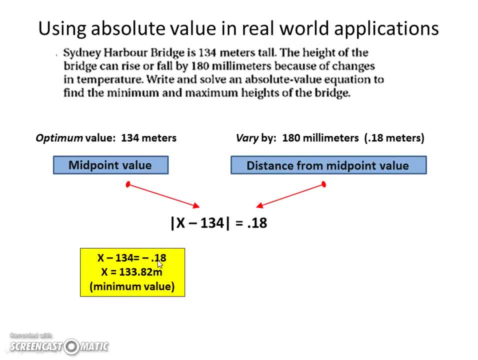 we allow it to vary by point 1- 8. so it we allow it to vary by point 1- 8. so it could be less point 1- 8 or more point 1 could be less point 1- 8 or more point 1. 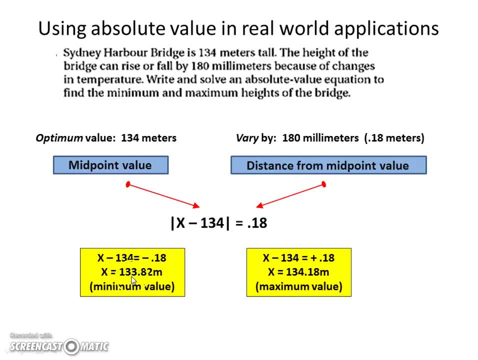 could be less point 1, 8 or more point 1: 8. if it's less, it's 134 minus 18 which 8. if it's less, it's 134 minus 18 which 8. if it's less, it's 134 minus 18, which gives us 133 point 82 meters. and if we 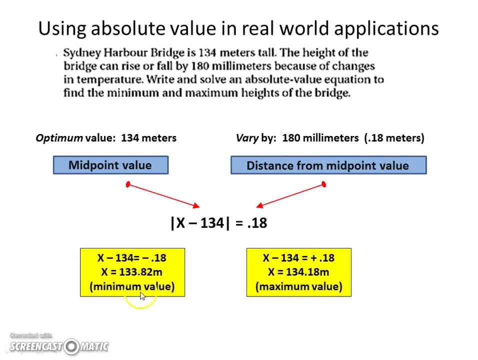 gives us 133 point 82 meters, and if we gives us 133 point 82 meters and if we add that point 18, it's 134 point 18. so add that point 18, it's 134 point 18. so add that point 18, it's 134 point 18. so there's our minimum value and our. 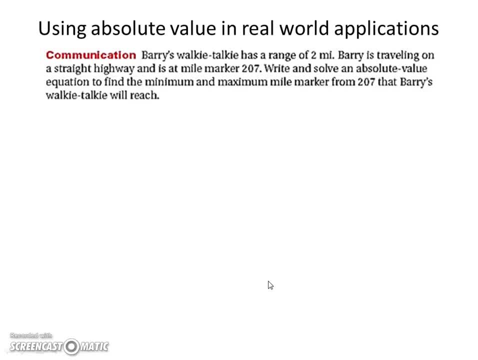 there's our minimum value and our. there's our minimum value and our maximum value. let's do a couple more in maximum value. let's do a couple more in maximum value. let's do a couple more in a different applications. okay, so here. a different applications. okay, so here. 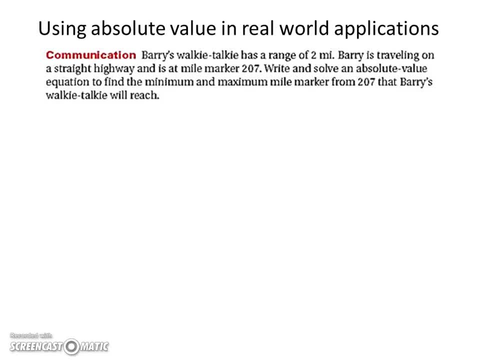 a different applications. okay, so here we're talking about Barry's walkie-talkie. we're talking about Barry's walkie-talkie has a range of two miles. Barry is has a range of two miles. Barry is has a range of two miles. Barry is traveling on a straight highway and is 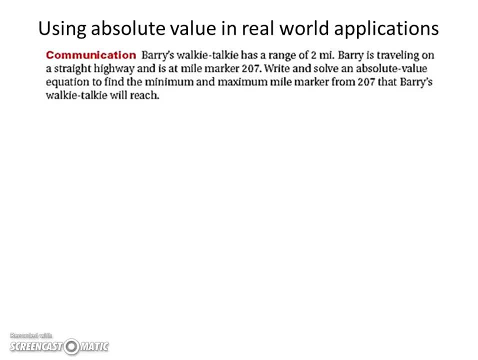 traveling on a straight highway and is traveling on a straight highway and is at mile marker 207 right and solve an at mile marker 207 right and solve an at mile marker 207 right and solve an absolute value equation to find the absolute value equation. to find the 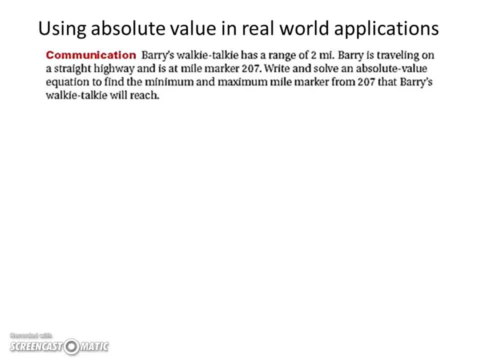 absolute value equation to find the minimum and maximum mile markers from 207. minimum and maximum mile markers from 207. minimum and maximum mile markers from 207 that Barry's walkie-talkie will reach, that Barry's walkie-talkie will reach, that Barry's walkie-talkie will reach, all right. so our midpoint value is 207. 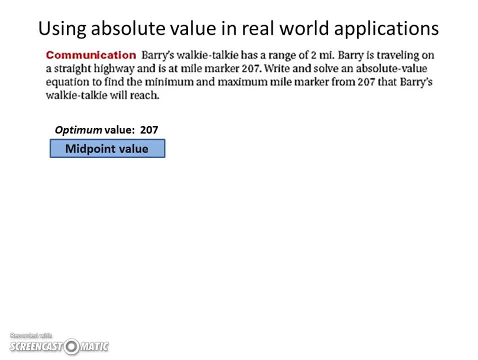 all right, so our midpoint value is 207. all right, so our midpoint value is 207. that's where Barry is. he's at marker 207. that's where Barry is. he's at marker 207. that's where Barry is. he's at marker 207 and we're allowing the range of the 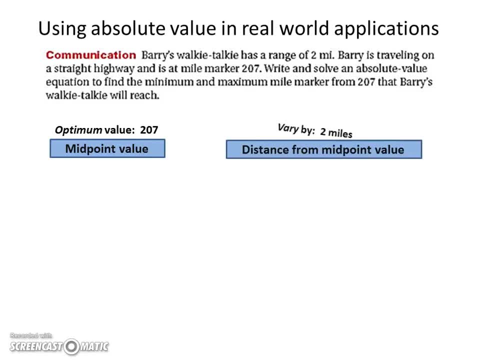 and we're allowing the range of the and we're allowing the range of the walkie-talkie to be two miles more, or walkie-talkie to be two miles more or walkie-talkie to be two miles more or less, so we're allowing it to vary by a. 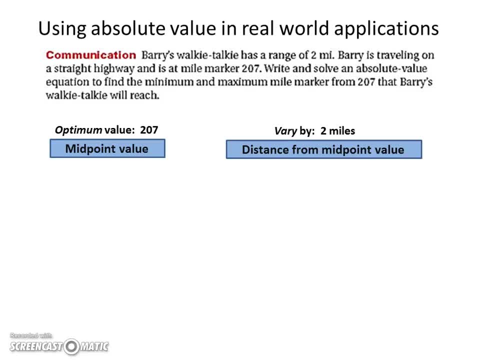 less. so we're allowing it to vary by a less, so we're allowing it to vary by a distance of two miles from that midpoint. distance of two miles from that midpoint. distance of two miles from that midpoint. value so our absolute value once again. value. so our absolute value once again. 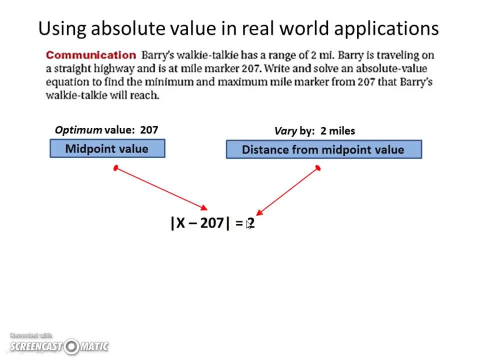 value. so our absolute value once again, 207 is what we want, but we're allowing value. so our absolute value once again, 207 is what we're allowing it to vary by. 207 is what we're allowing it to vary by. 207 is what we're allowing it to vary by two- two more or two less, so two less. 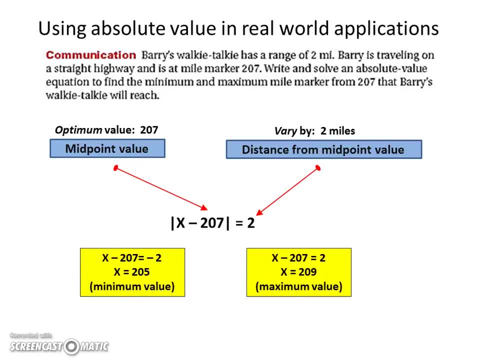 two, two more or two less. so two less. two, two more or two less. so two less would be 205, two more would be 209. look would be 205. two more would be 209. look would be 205. two more would be 209. look at one more. a little bit of a problem. 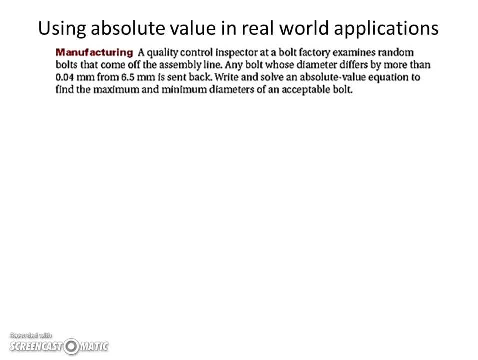 at one more a little bit of a problem. at one more a little bit of a problem with manufacturing: a quality control with manufacturing. a quality control with manufacturing. a quality control. inspector at a bolt factory examines. inspector at a bolt factory examines. inspector at a bolt factory examines random bolts that come off the assembly. 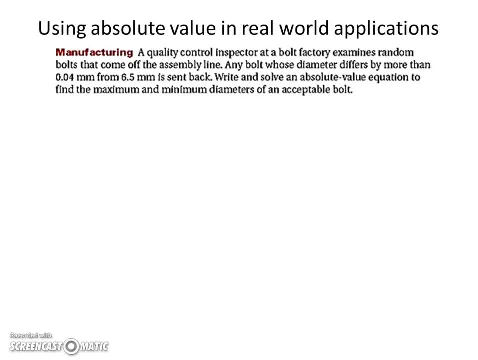 random bolts that come off the assembly. random bolts that come off the assembly line: okay. so his job is to check to make line. okay, so his job is to check to make line. okay, so his job is to check to make sure that the bolts are within a certain 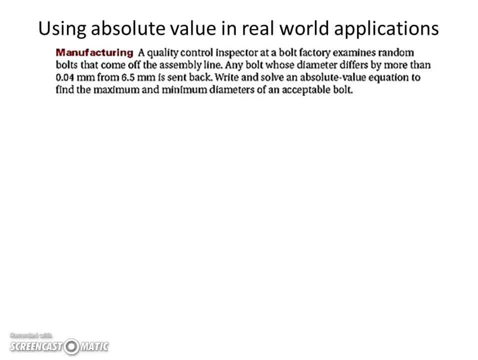 sure that the bolts are within a certain sure that the bolts are within a certain size. if they're too big or too small size, if they're too big or too small size, if they're too big or too small, they have to be thrown out. so any bolt. 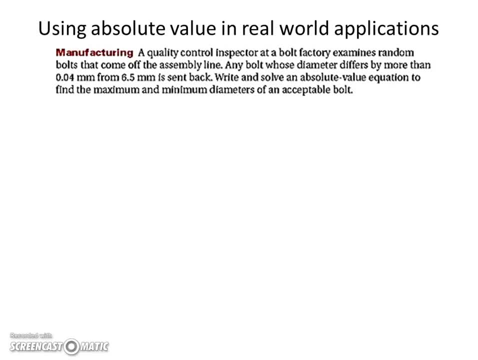 they have to be thrown out. so any bolt. they have to be thrown out. so any bolt whose diameter differs by more than 0.04, whose diameter differs by more than 0.04, whose diameter differs by more than 0.04 millimeters from 6.5 millimeters is sent. 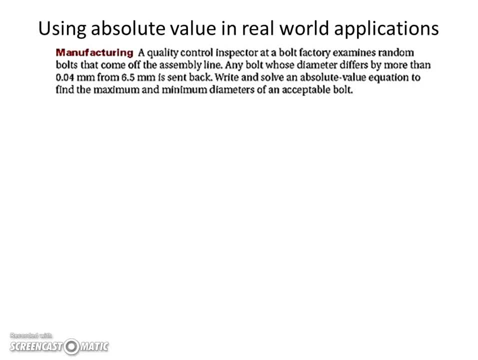 millimeters from 6.5 millimeters is sent, millimeters from 6.5 millimeters is sent back. they have to remake them. okay, write back. they have to remake them. okay, write back. they have to remake them. okay, write and solve an absolute value equation to: 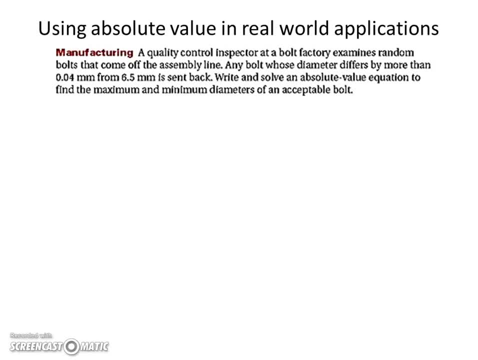 and solve an absolute value equation to and solve an absolute value equation to find the maximum and minimum diameters. find the maximum and minimum diameters. find the maximum and minimum diameters of an acceptable boat. okay, so once again. of an acceptable boat. okay, so once again. 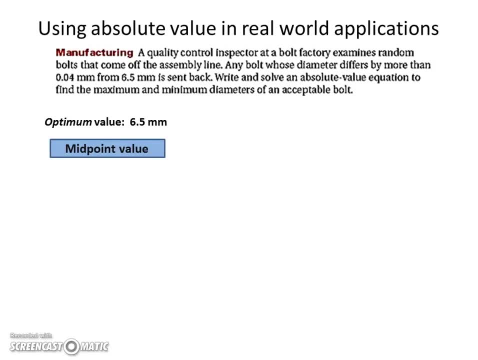 of an acceptable boat. okay, so once again, we want 6.5 millimeters. that's how much we want 6.5 millimeters. that's how much we want. 6.5 millimeters. that's how much we want the diameter to be. but we're. 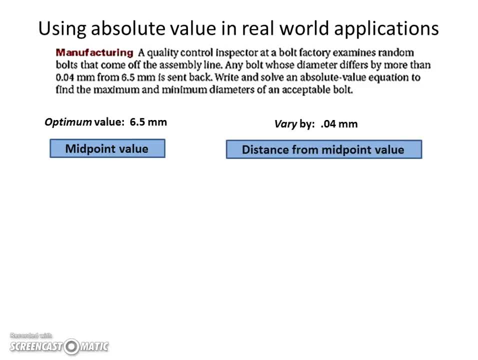 we want the diameter to be, but we're. we want the diameter to be, but we're allowing it to vary by as little as point, allowing it to vary by as little as point, allowing it to vary by as little as point. 0, 4 millimeters, it's not a lot. but 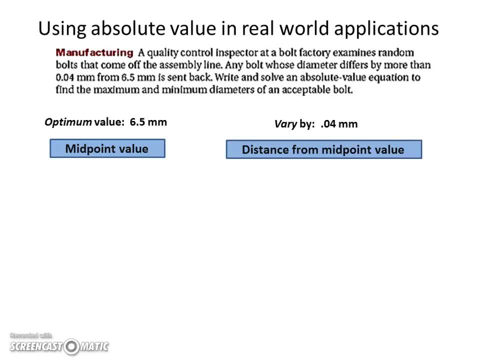 0, 4 millimeters, it's not a lot. but 0, 4 millimeters, it's not a lot, but that's you have to be pretty exact when that's. you have to be pretty exact when that's. you have to be pretty exact when you're talking about creating a bolt or 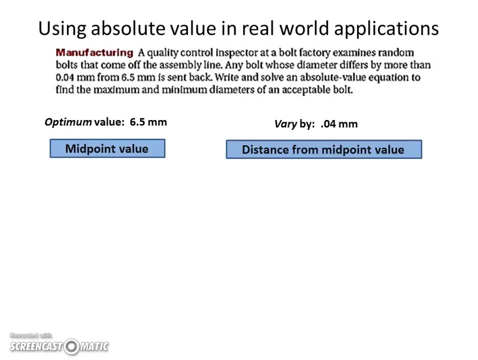 you're talking about creating a bolt, or you're talking about creating a bolt or something that's small, so we're allowing something that's small. so we're allowing something that's small, so we're allowing it to be 0.04 millimeters bigger, or? 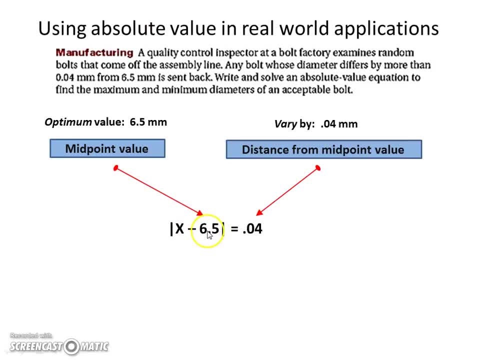 it to be 0.04 millimeters bigger, or it to be 0.04 millimeters bigger or smaller. so once again, we want it to be smaller. so once again, we want it to be smaller. so once again, we want it to be 6.5, but we're allowing it to vary by. 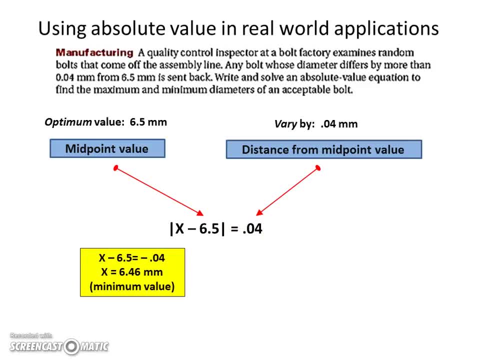 6.5, but we're allowing it to vary by 6.5, but we're allowing it to vary by 0.04. so we can either take away that 0.04, so we can either take away that 0.04. so we can either take away that point 0: 4 or we can add the point 0: 4. point 0: 4. or we can add the point 0: 4. point 0: 4 or we can add the point 0: 4. there's our Mac minimum value 6.4- 6. there's our Mac minimum value 6.4, 6. 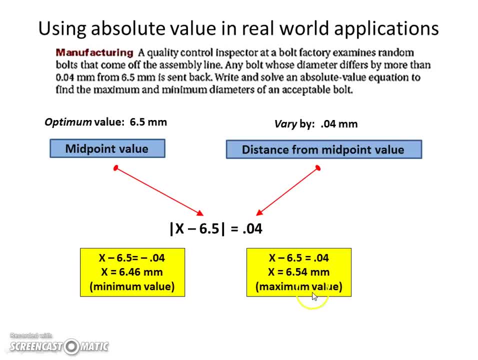 there's our Mac minimum value 6.4, 6 millimeters and our maximum value would millimeters and our maximum value would millimeters and our maximum value would be 6.5, 4 millimeters. that's it gives you be 6.5, 4 millimeters. that's it gives you. 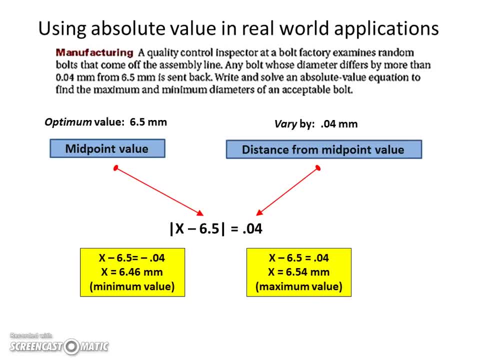 be 6.5, 4 millimeters. that's, it gives you some idea of how we can solve these, some idea of how we can solve these, some idea of how we can solve these problems. if you need a, if you have any problems, if you need a, if you have any. 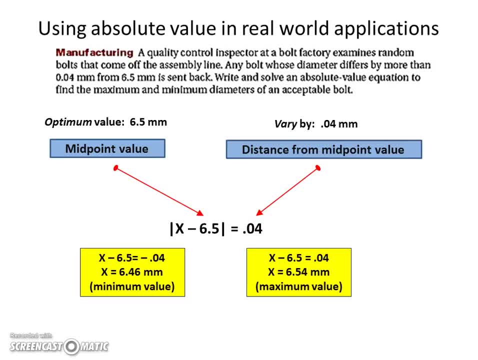 problems. if you need a, if you have any questions, feel free to email me or bring questions. feel free to email me or bring questions. feel free to email me or bring up your questions in class. see you soon up your questions in class. see you soon up your questions in class. see you soon, bye.